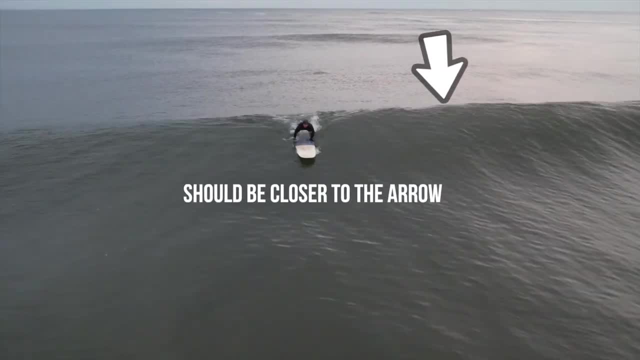 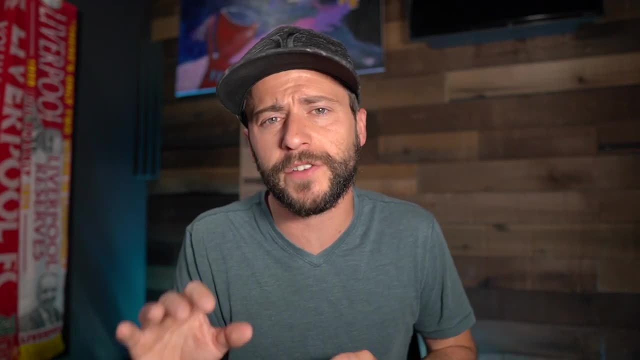 wave too far out on the shoulder, you're probably not going to catch the wave at all. If you're catching the wave too deep, it's most likely going to close out in front of you To put yourself in the perfect spot. you have to understand how waves work and also what to 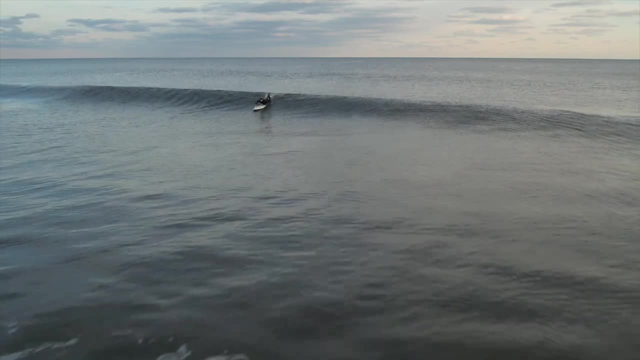 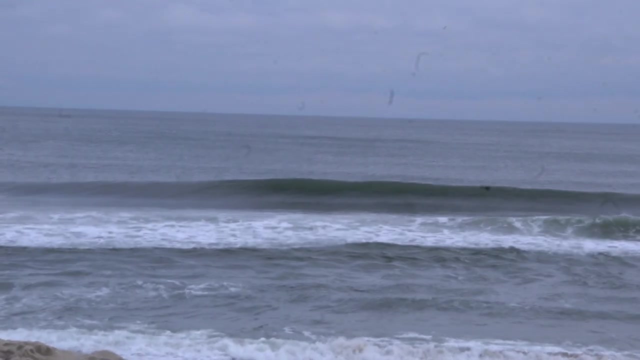 look for When you're looking at a wave. one of the most important aspects is the peak. This is the point on the face of the wave that's the tallest and is going to break first. In a perfect world, we would try to take off at the peak and decide whether we're going. 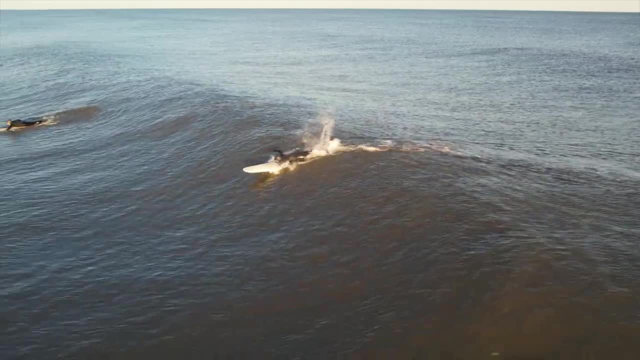 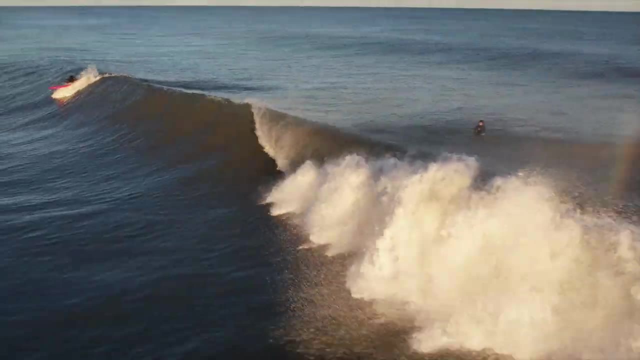 to go right or left, depending on what the shoulder looks like. However, waves are rarely perfect. In this scenario, I took off at the peak when, in reality, the spot to take off was between me and Gilad. I gained this knowledge by wiping out, and now I'll be looking to. 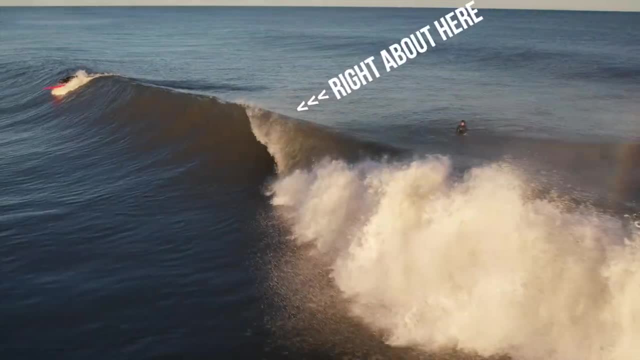 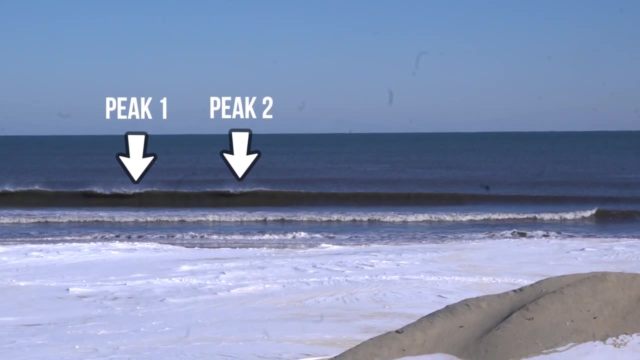 take off 15 yards or so to the right of the peak the rest of the session. Ideally, you should be taking off as close to the peak as you can, while avoiding the closeout sections. The closer you are to the peak or the steeper part of the wave, the easier the wave is. 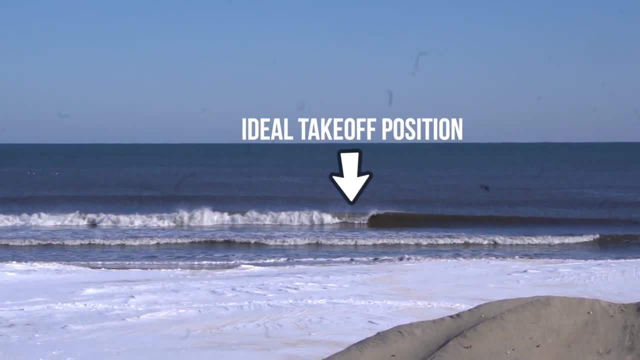 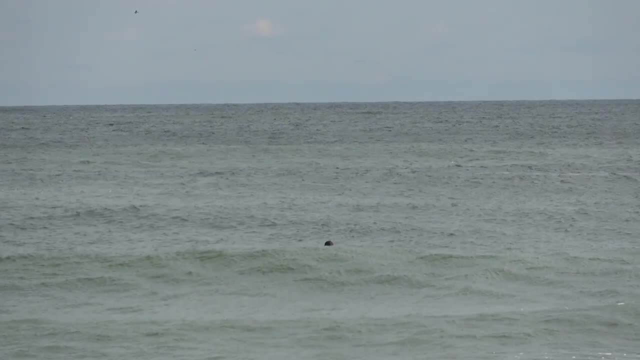 to catch Now. as discussed in the first tip, you should be studying the waves before you paddle out, just to get an idea of how they're breaking. However, the ocean is constantly changing, so you have to learn how to adapt on the fly. This is why you always see the 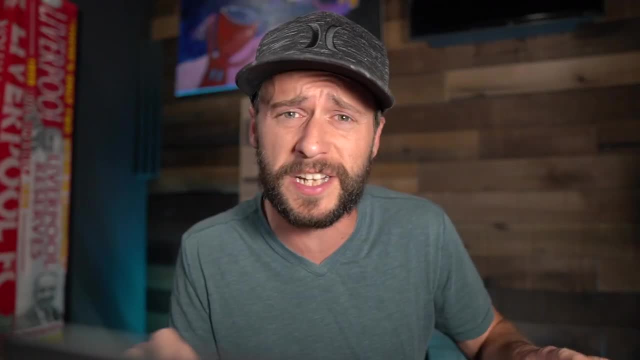 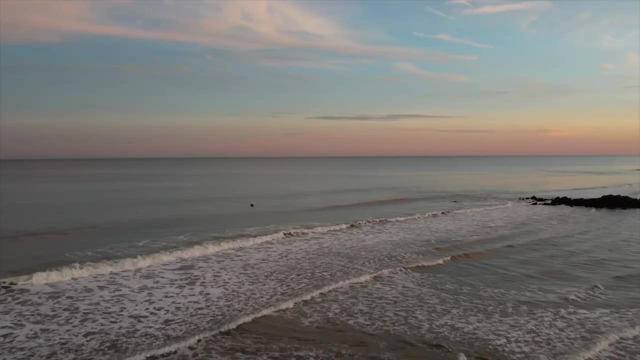 best surfers, constantly paddling for position and rarely sitting still for extended periods. While we're sitting waiting for waves, especially at beach breaks, you have to constantly be scanning the ocean If you're looking for bumps. those bumps can give us an indication that a wave might. 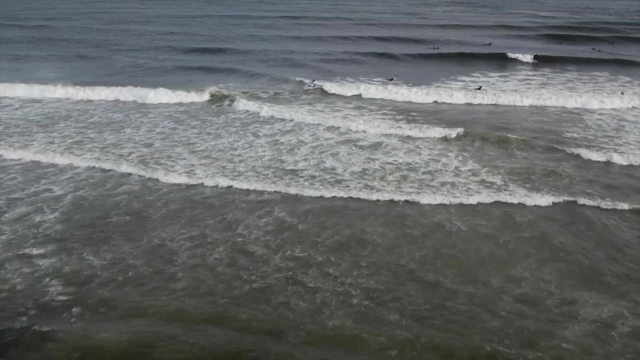 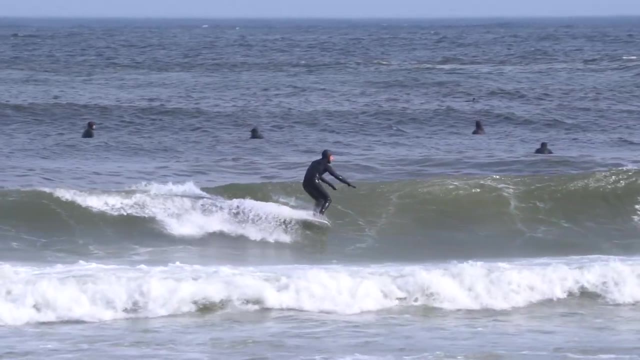 be coming. Have you ever noticed those times where every surfer is just sitting and waiting for a wave and then, all of a sudden, everyone drops to their boards and starts paddling in unison? That's because they all saw a bump. If I see a bump, that's about this wide. 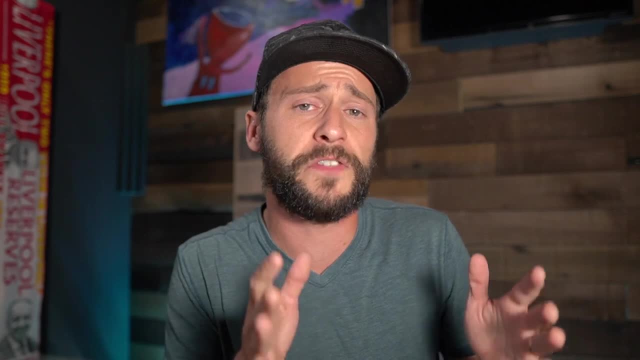 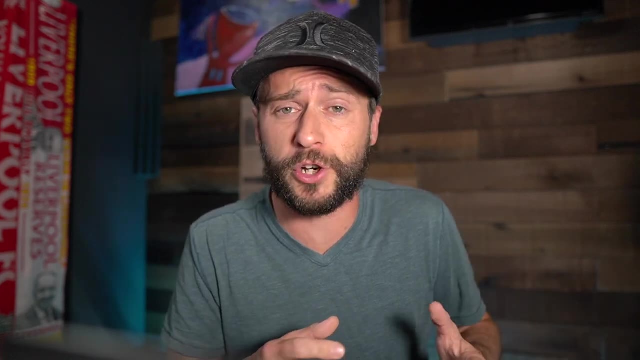 and I'm looking to catch the wave. about 15 yards to the right of the peak. you'll see me start to paddle towards that spot well before the wave ever gets to me. Sometimes I'll see a bump. I'll paddle towards it and it'll turn out to be absolutely nothing. 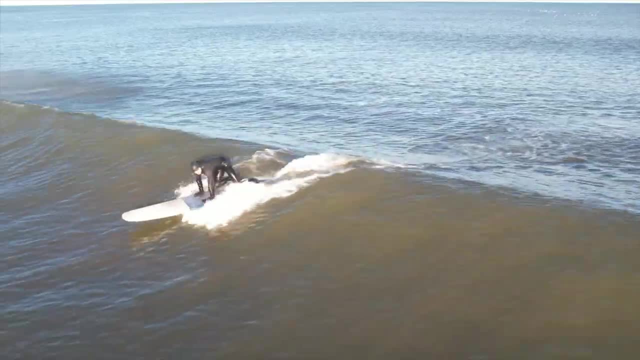 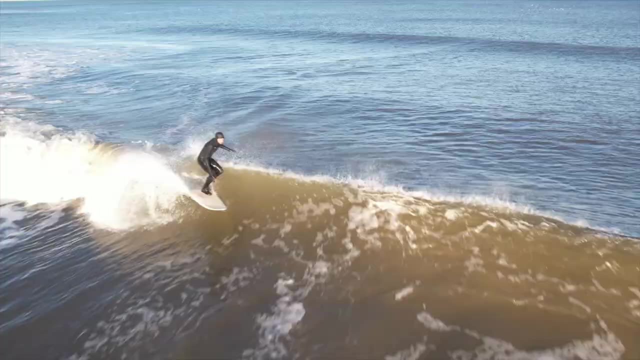 and that's surfing, Constantly, scanning, paddling, getting it right, sometimes failing miserably. sometimes, The more time you spend in the water focusing on these things, the better your positioning is going to get. And finally, mistake number three- and the most common among new surfers- is not paying.